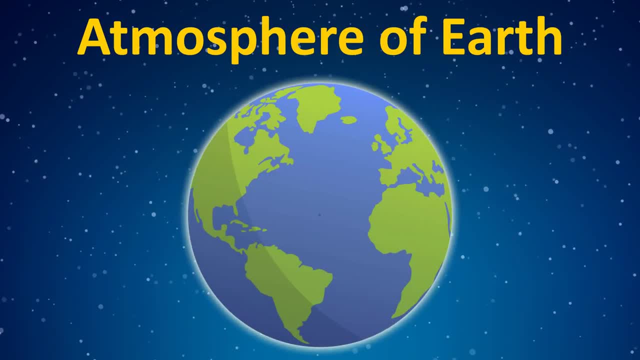 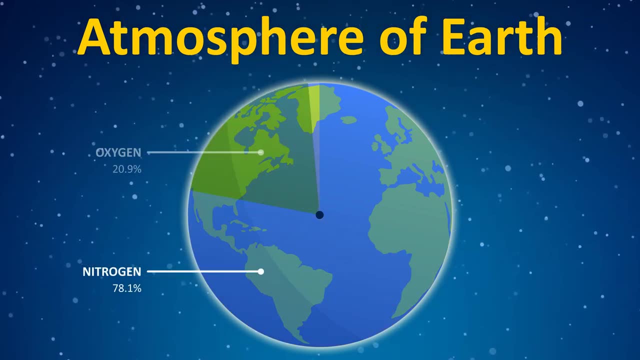 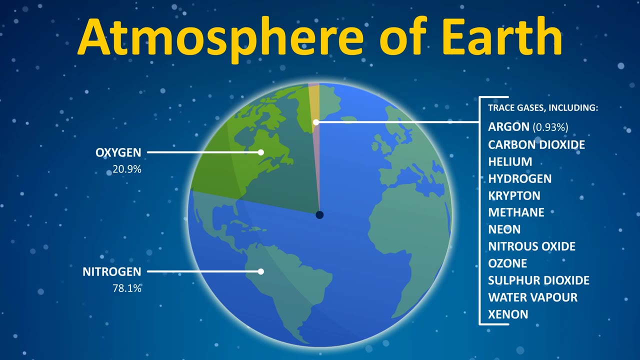 What is Earth's atmosphere? Earth is surrounded by its atmosphere, which is the body of air or gases that protects the planet and enables life. The three major constituents are nitrogen, oxygen and argon. Earth's atmosphere has five distinct layers. Let's look at each from closest to. 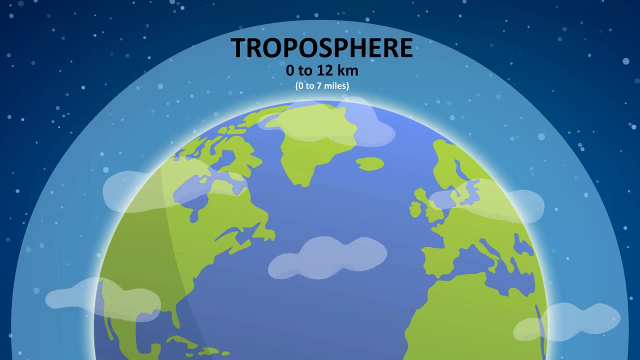 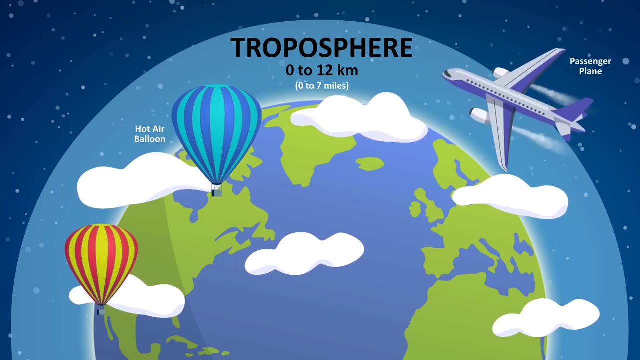 farthest from the Earth- Troposphere. The layer of the atmosphere closest to the Earth is the troposphere. It begins at the surface of the Earth and extends out to about 12 kilometers. This layer is known as the lower atmosphere. It's where weather happens and contains the 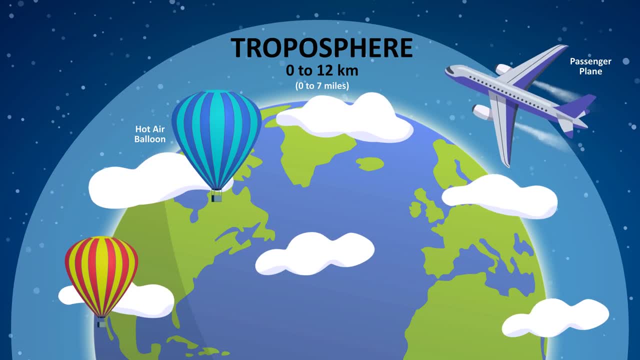 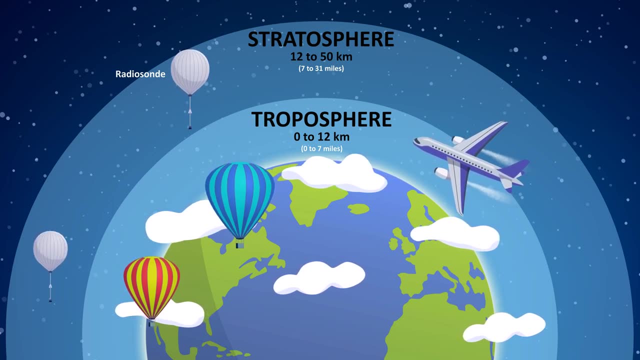 air humans breathe. The temperature of the troposphere decreases with height. Stratosphere- Above the troposphere is the stratosphere. This layer is where the ozone layer exists and scientists send weather balloons. Jets fly in the lower stratosphere to avoid. 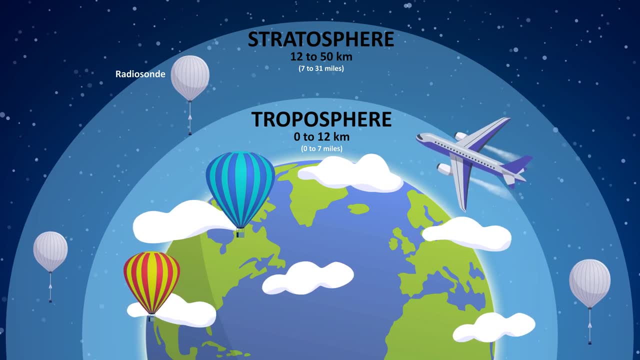 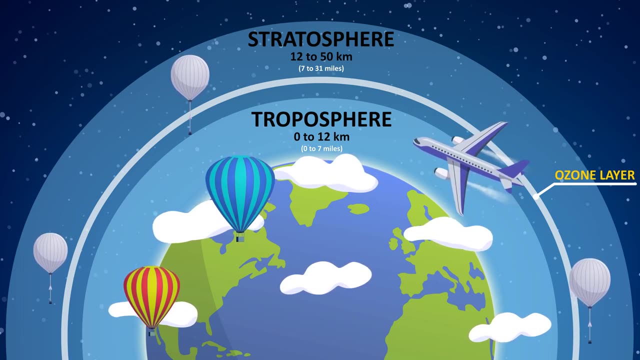 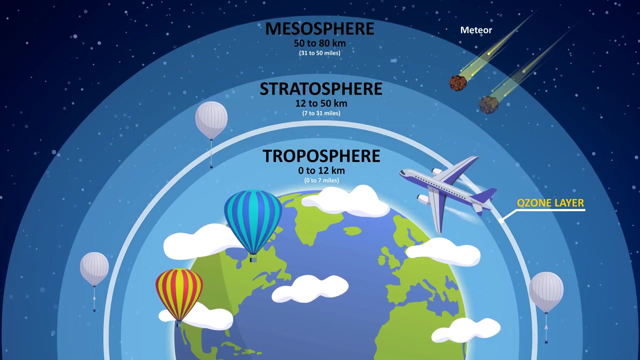 turbulence in the troposphere. Temperature rises within the stratosphere but still remains well below freezing Ozone layer. The ozone layer is a region of Earth's stratosphere that absorbs most of the sun's ultraviolet radiation. Mesosphere, The layer where the air is especially thin and molecules are great distances apart, is 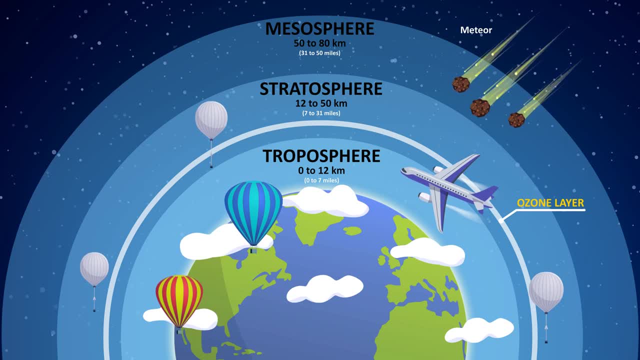 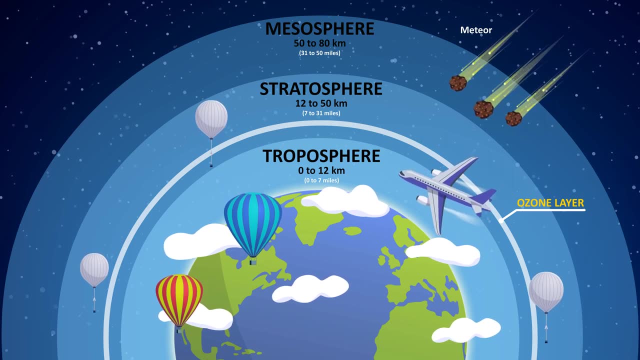 the mesosphere. Temperatures in the mesosphere reach a low of minus 90 degrees Celsius. Meteors burn up in this layer. The stratosphere and the mesosphere are known as the middle atmospheres Thermosphere. The thermosphere rises several hundred kilometers above the Earth's surface. 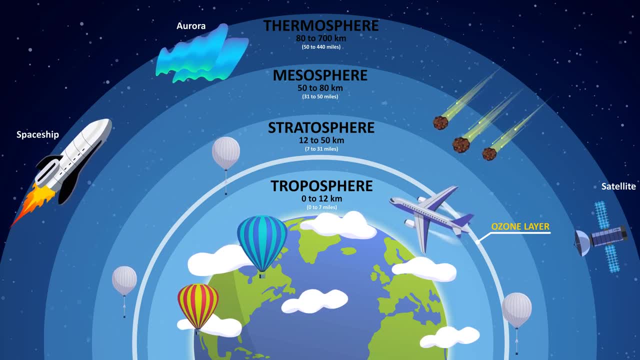 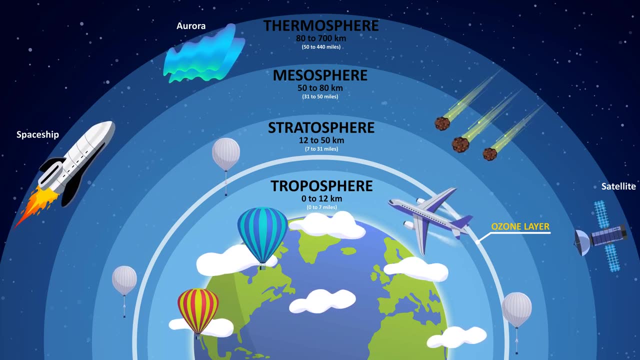 Temperature is very much affected by the sun. here. Temperature increases with height and can rise to as high as 2,000 degrees Celsius. Nonetheless, the air would feel cold because the hot molecules are so far apart. Karman line: The Karman line is based on physical reality in the sense that it 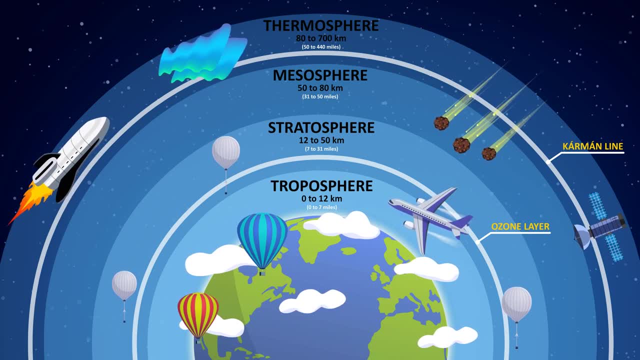 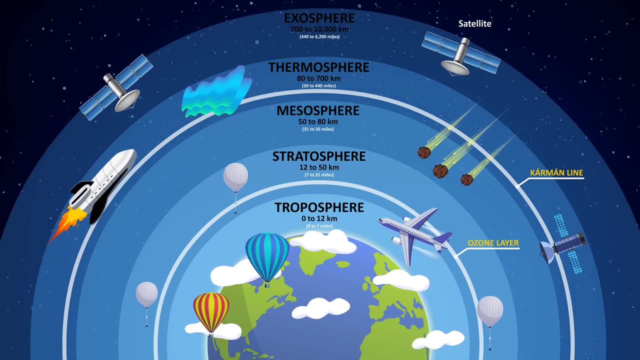 roughly marks the altitude where traditional aircraft can no longer effectively fly. Exosphere- The exosphere has very few atmospheres. The exosphere has very few atmospheres. The exosphere has very few atmospheric molecules which can escape into space. Some scientists disagree that the exosphere 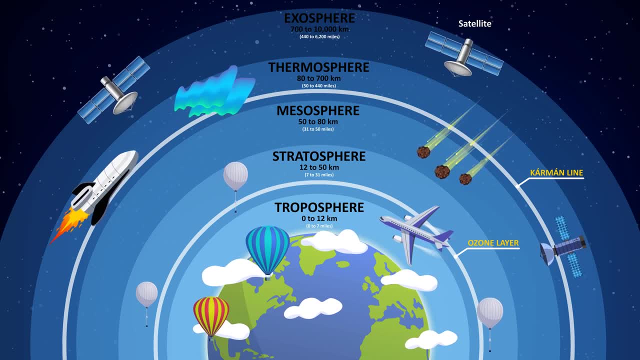 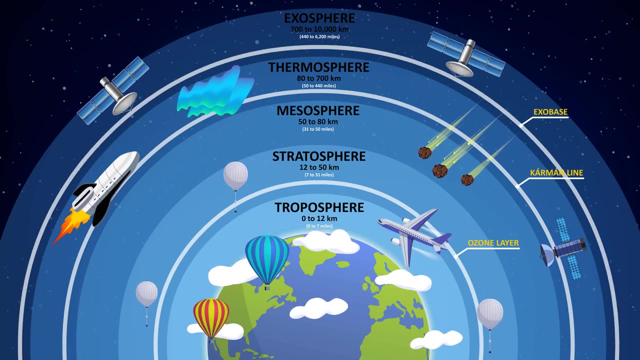 is a part of the atmosphere and instead classify it actually as a part of outer space. There is no clear upper boundary as in other layers. Exobase, The lower boundary of the exosphere is called the exobase. It is also called the critical altitude, as this is the altitude where barometric conditions